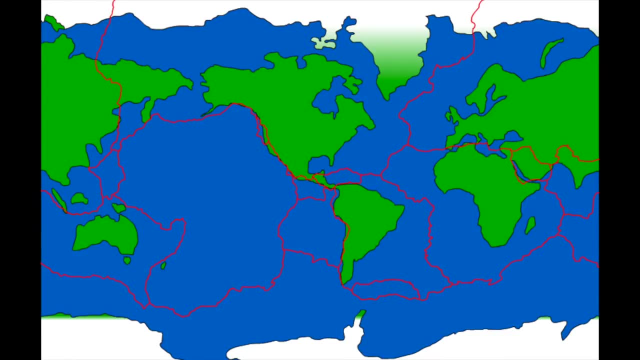 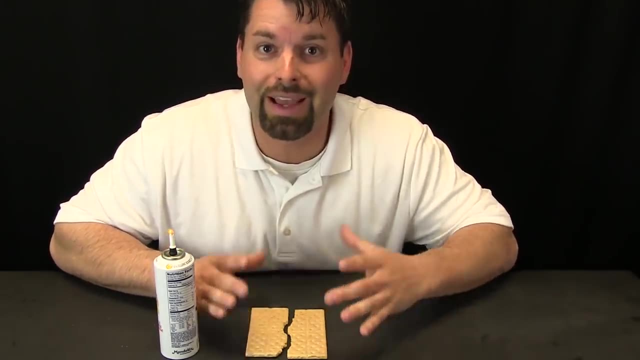 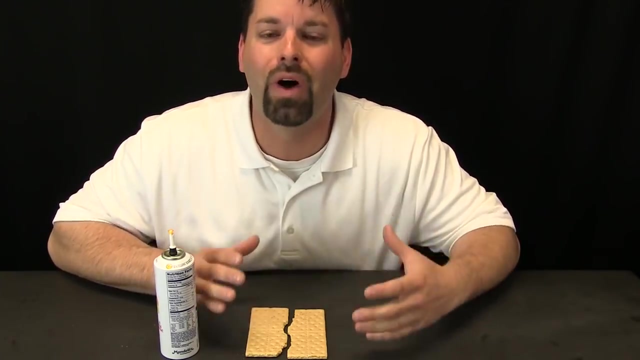 The crust is actually broken into pieces or plates. It is not just one. There are many pieces or plates. Through science, we have discovered that all those pieces and plates actually move. Now, in another video, we talked about why those plates move. Today we want to talk about what happens when those plates move. 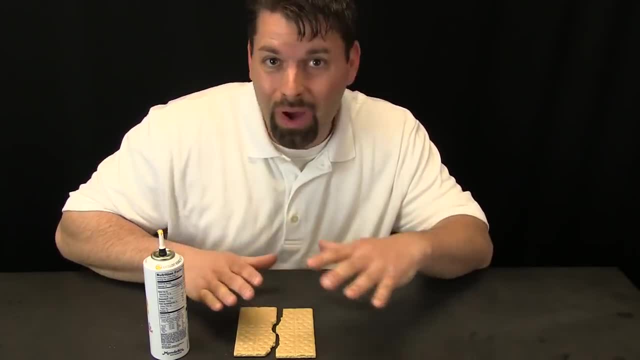 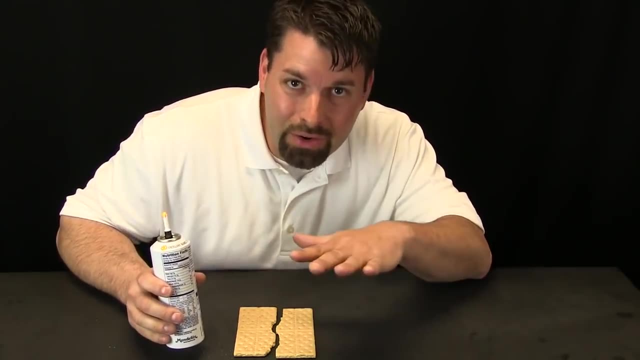 So we are going to zoom in and take a closer look so you can see what happens when those plates move. But to do that, to show you that, we are going to use spray cheese to lay down the mantle right under the crust And then we are going to use graham crackers to be the crust. 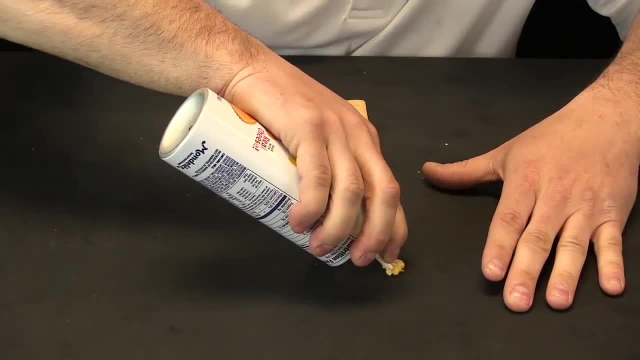 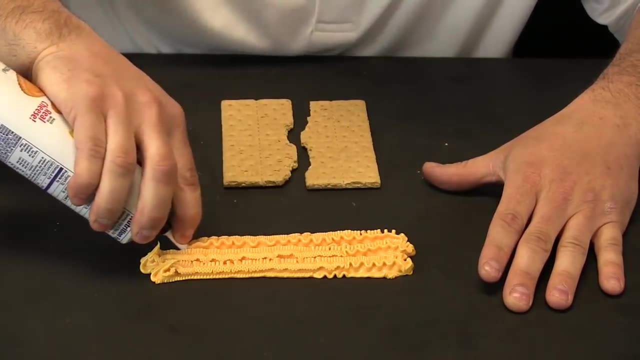 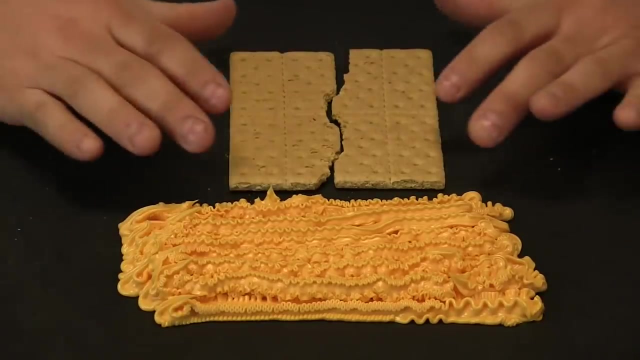 So first we need to lay down the mantle, the part right under the crust, And to do that I am just going to spray some of this cheese. It is important to remember that this mantle is hot and parts of the mantle are moving. 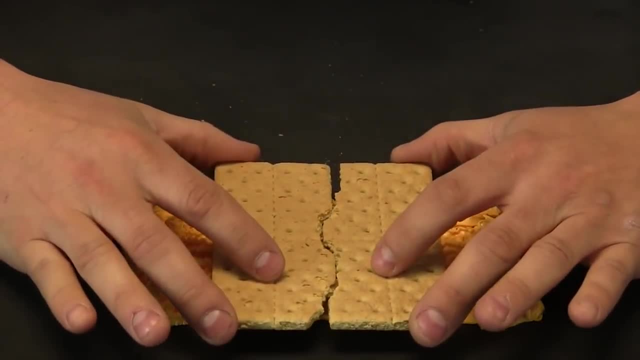 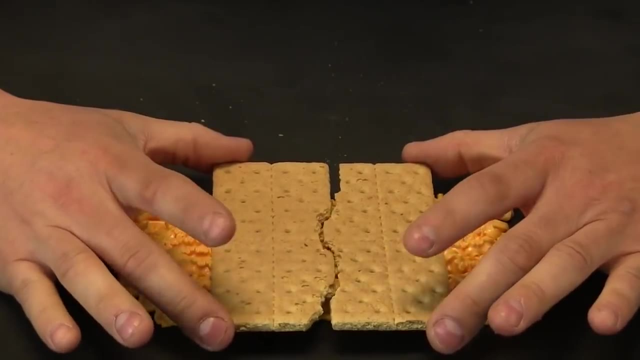 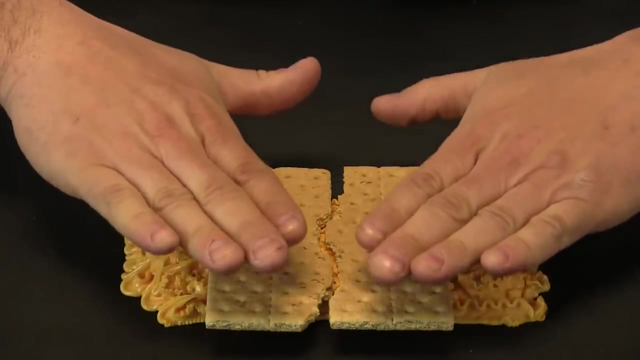 And then we have the crust. The crust sits on top of the mantle in pieces or plates, And because parts of the mantle are moving, that means parts of my crust are moving, And that is what we want to look at. Remember that continents and oceans are sitting on top of this crust. 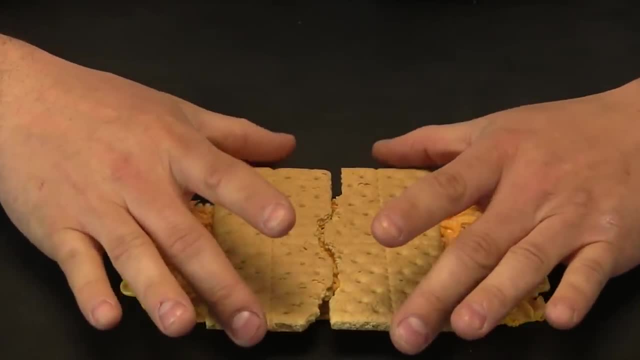 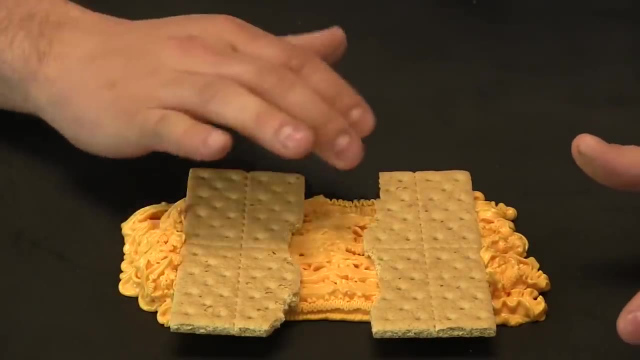 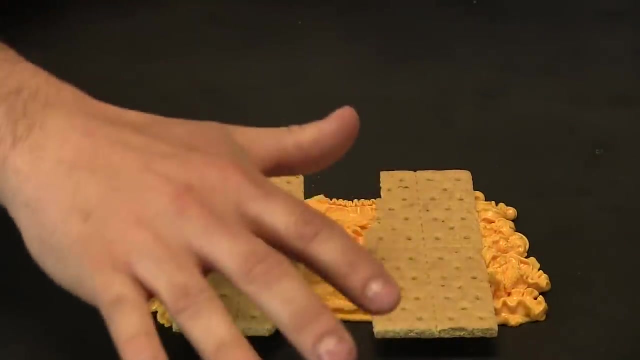 And those plates are moving. And one way those plates can move is those plates can actually move apart. When they move apart, that mantle actually forms new crust. And when the plates move apart, this is happening under the ocean. Actually, new crust is added as those plates move apart. 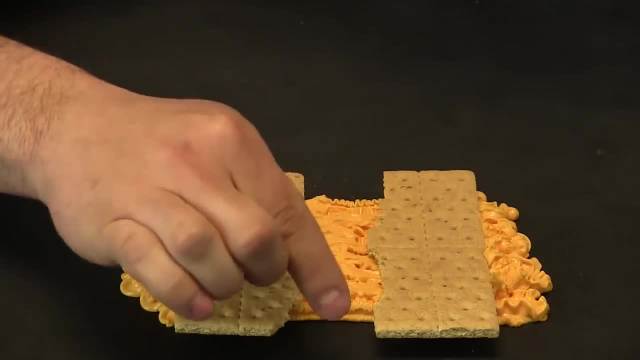 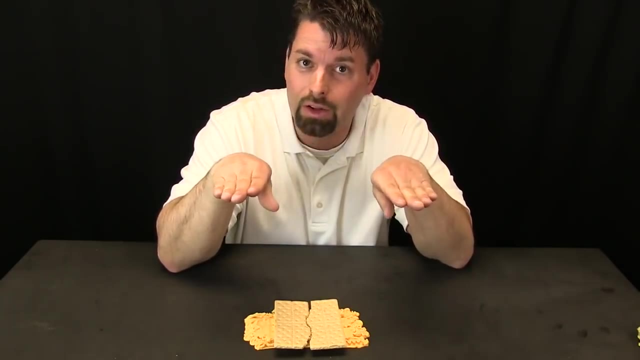 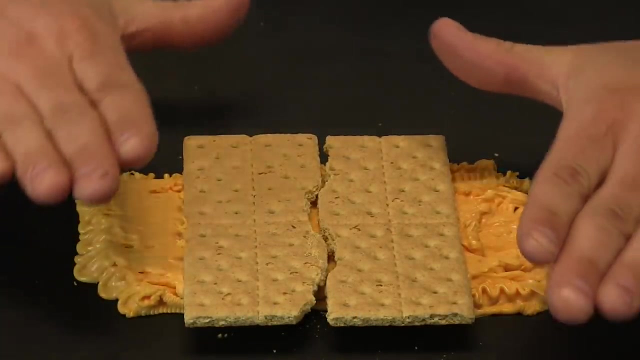 And right here, as the plates move apart, the mantle cools down and it forms new crust. So we have seen that plates can actually move apart. But let us take a closer look at what happens when plates slide past each other. Okay, so we have zoomed in so we can take a closer look at what happens when the plates slide past each other. 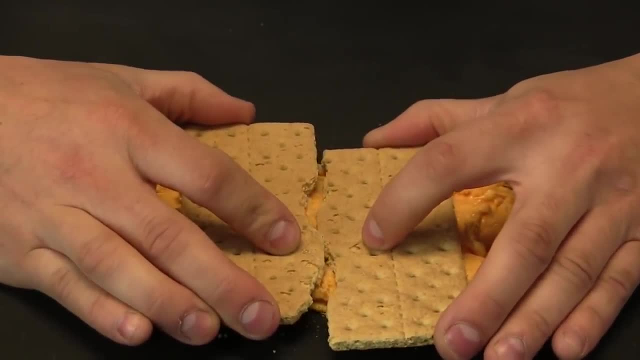 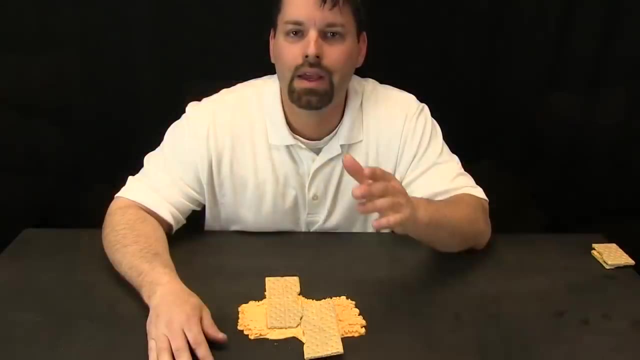 Watch what happens as I slide the plates past each other. It is important to remember It is not a smooth ride. It is actually quite bumpy. In fact, that bumpy ride as plates slide past each other, that is what creates earthquakes. 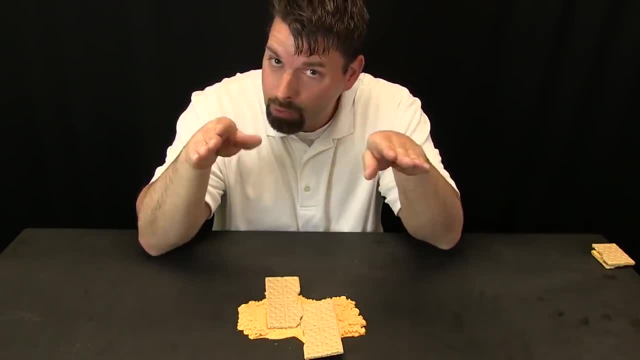 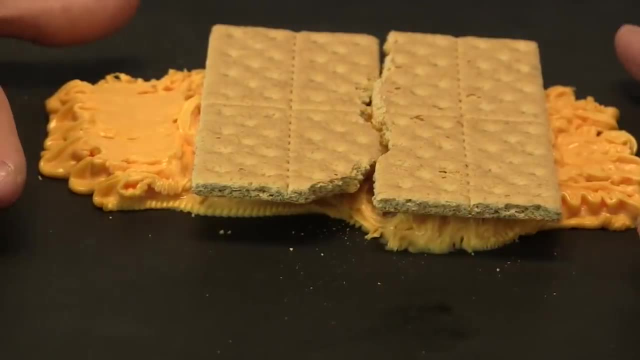 So we have talked about what happens when plates move apart and what happens when plates move past each other. Well, what happens when plates bump into each other? So we have zoomed in again to see what happens when one plate collides with another.